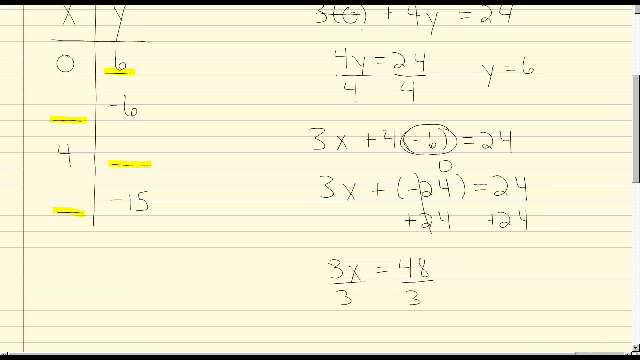 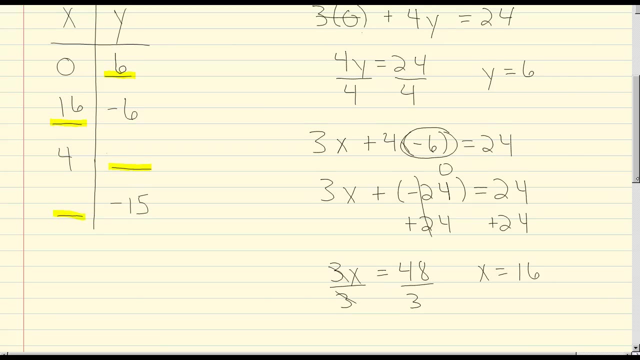 of the equation by 3, so that we can solve for x. And so we're going to get x equals 16.. Okay, so we're going to fill in our x value over here with a 16.. Alright, our next given value is a 4 for x, So we're going to plug in a negative 6 for y. So we're going. 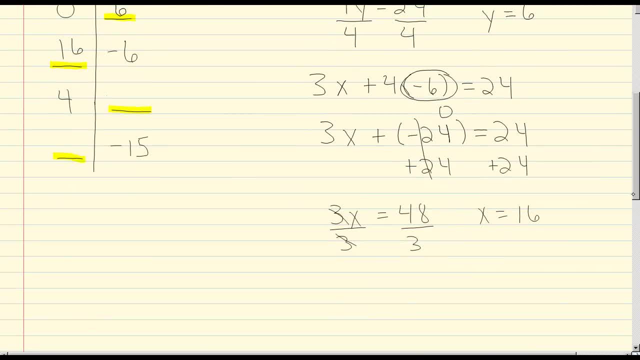 to plug in a 4 for the x. Let me just rewrite the equation down here: 3x plus 4y equals 24.. Okay, so we're going to be plugging in a 4 for the x and we're going to solve for. 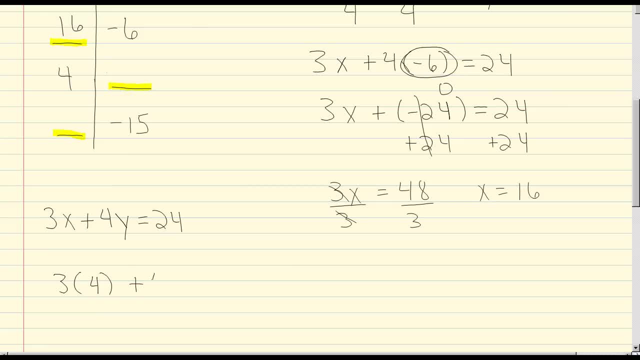 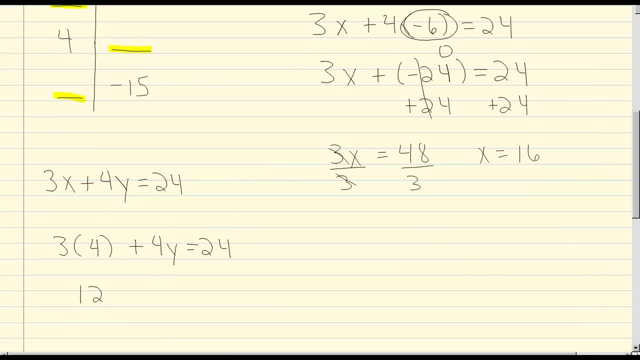 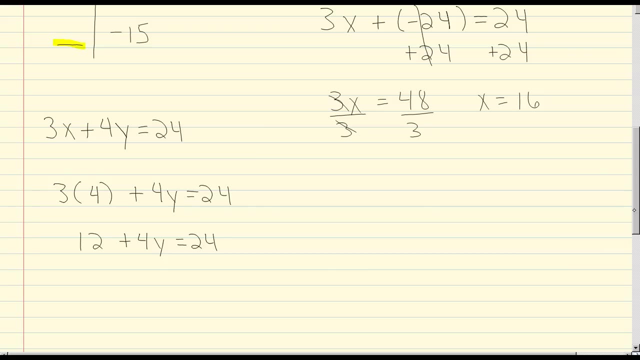 y. So we'll have 3 times 4 plus 4y equals 24.. Okay, 3 times 4 is 12.. So you'll have 12 plus 4y equals 24.. Alright, we're going to subtract 12 from both sides of the equation. 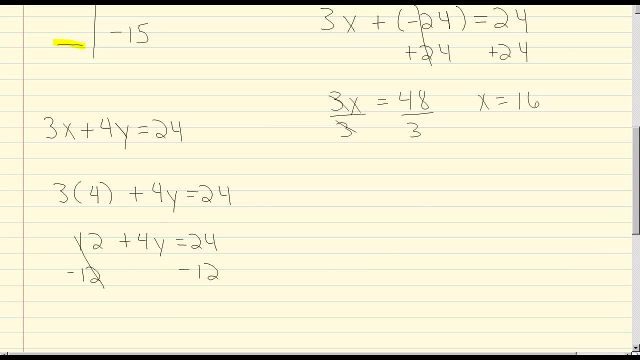 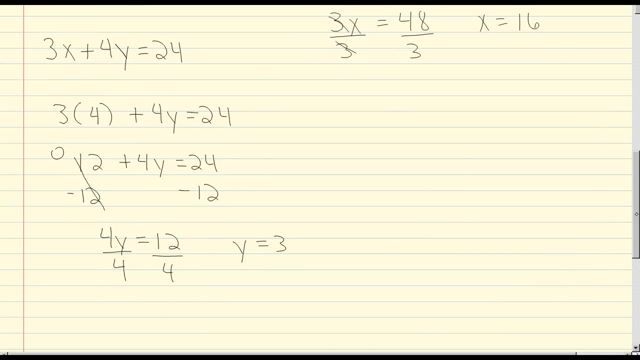 That'll be 0.. 24 minus 12 is 12.. So this will be 4y equals 12. And we can just divide both sides of the equation by 4. And so we'll get y equals 3.. Okay, so we'll come back up. 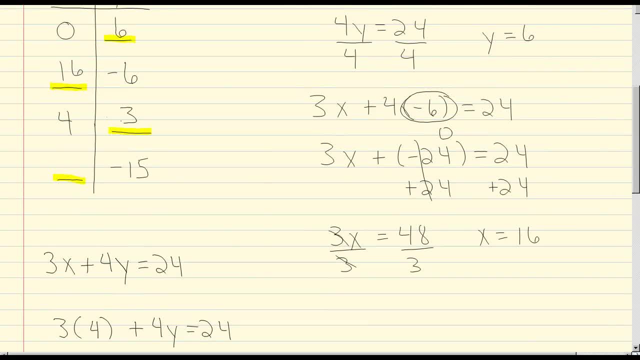 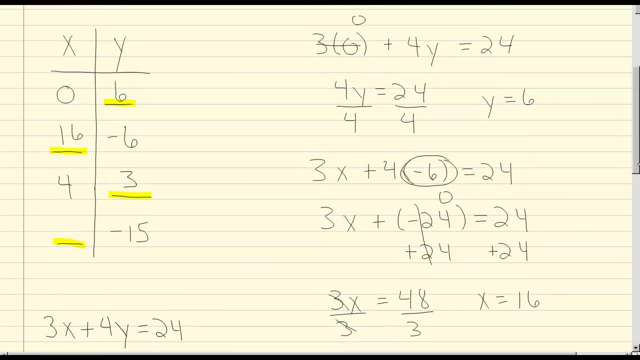 here and fill this in as a 3.. Alright, so when x equals 4, y is going to be 3.. Alright, so our final given value is a negative 15 for x. Alright, so we're going to plug in. 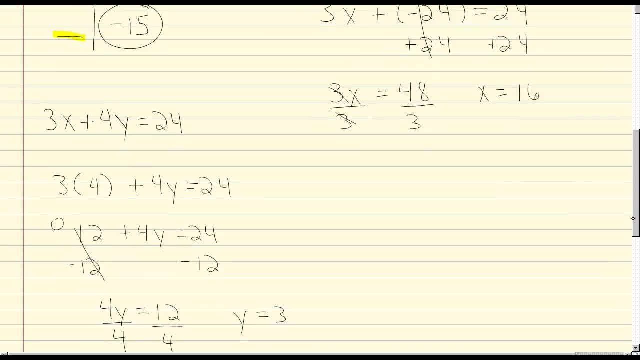 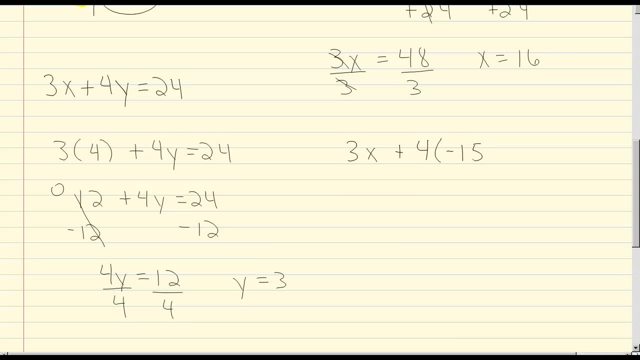 a negative 15 for y. So let's go back down here and plug in a negative 15 for y. So we'll have 3x plus 4 times negative 15. And this should be equal to 24.. Okay, 4 times negative. 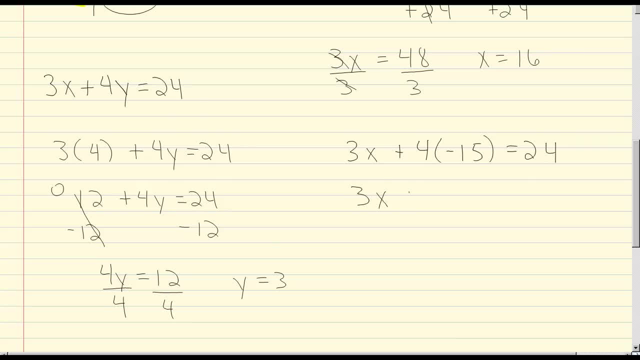 15 is negative 60. So we'll have 3x plus negative. 60 equals 24.. Add 60 to both sides of the equation. That'll be 0.. 24 plus 60 equals 24.. Alright, so we're going to plug in a negative. 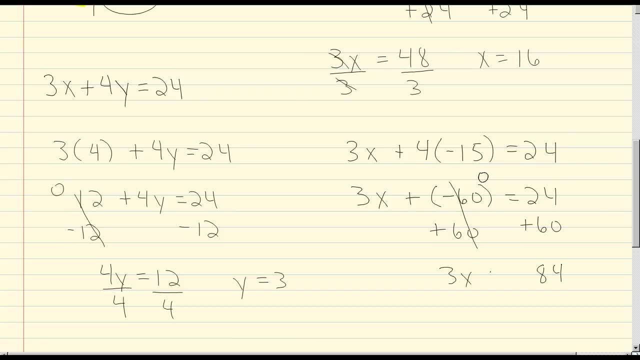 25 for y. So this is our final given value, 8.ungspeattlenet plat. So the last percent we need is 84. So we'll have 3x equals 84. And so we're going to just divide both sides.